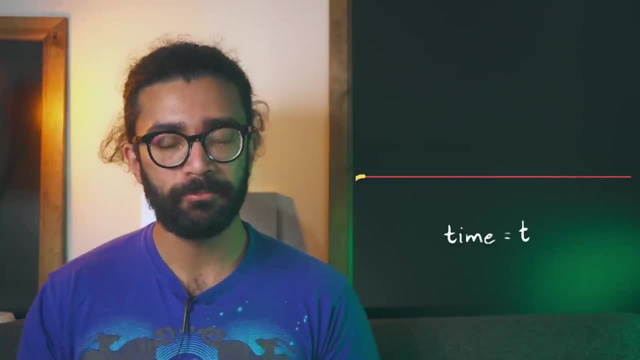 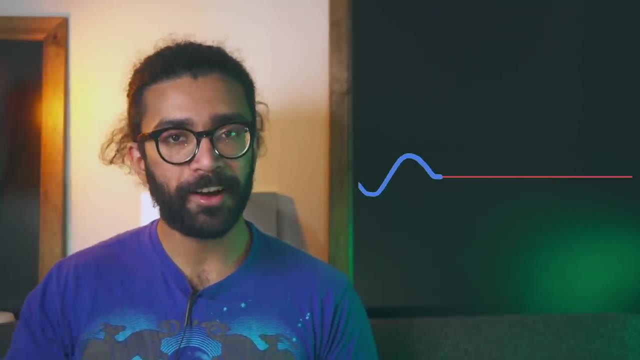 the string looks like this, and then, at a later value of t, the string looks like this: Now let's imagine another wave coming the other way. Maybe we set this one up by plucking the other side of the string. What happens when these two waves arrive at the same part of the string? 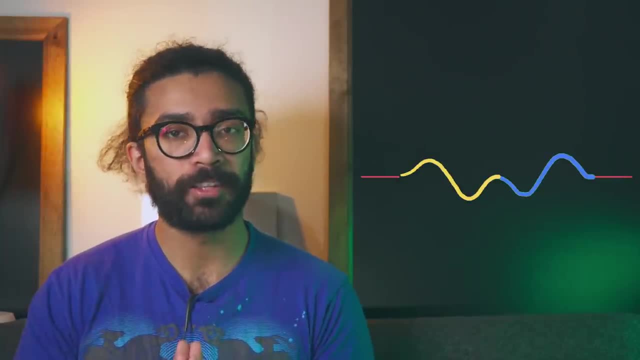 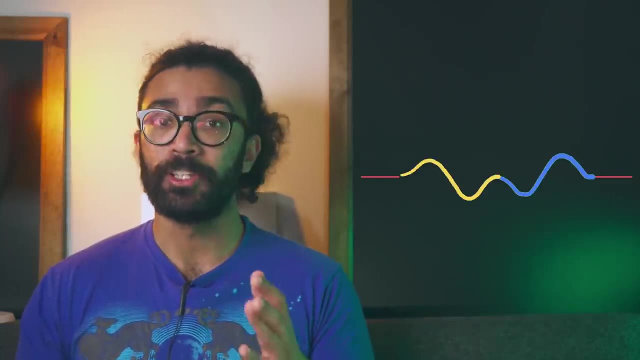 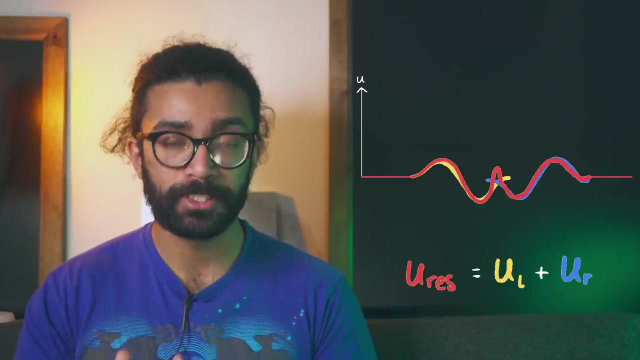 Well, common sense suggests that the wave that we end up seeing on the string is a combination of the two original waves. We can take the value of u for each wave at each point in space and at each point in time and simply add them up to give us the resultant wave, And this is actually what ends. 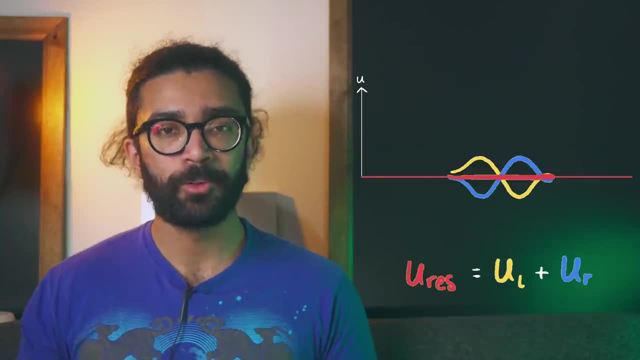 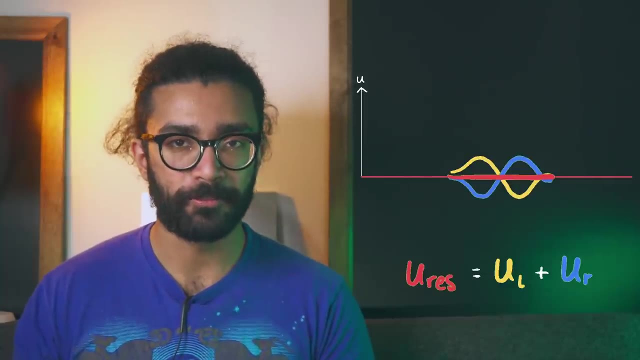 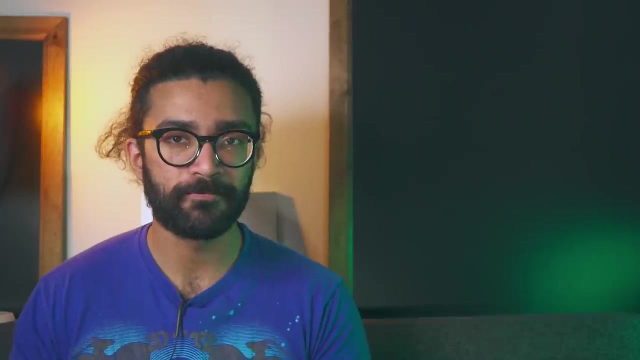 up happening When waves are moving, so that they overlap. we end up adding their displacements at each point in space and time to give us the overall resultant wave. But common sense is not always right. So can we work out why this time it works Well, one way to think about this is that 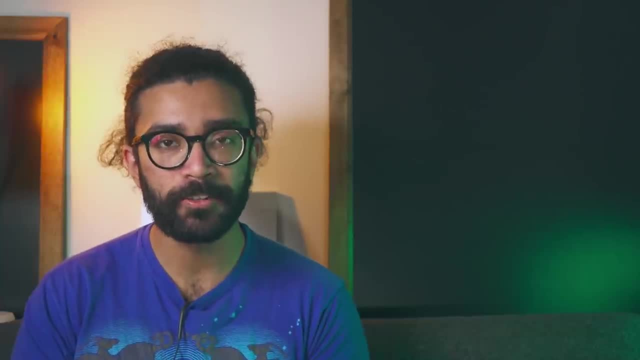 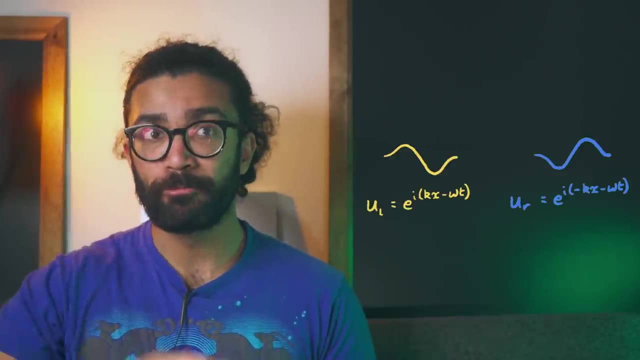 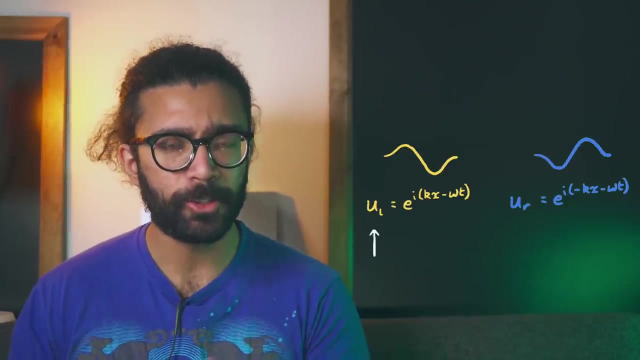 the equations which dictate how waves should behave are known as linear equations. Let's see what this means. First of all, we can represent either of our original waves as mathematical functions through space and over time. All this tells us is the value of u for every given x position and, at every time, value t. 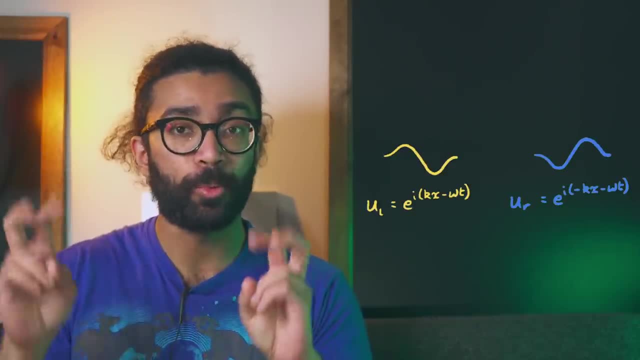 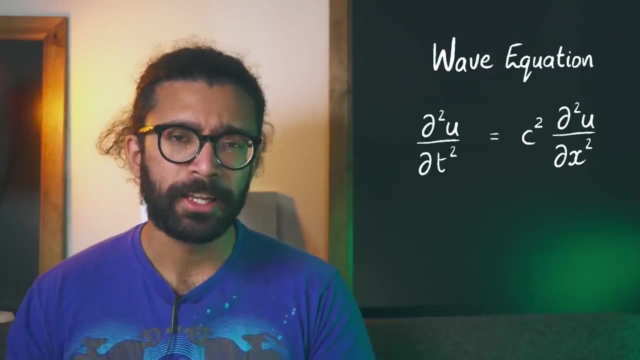 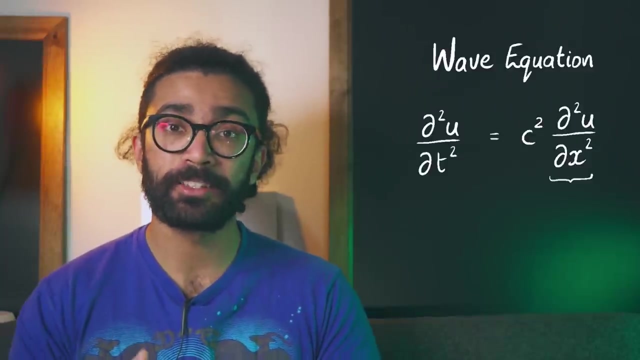 Then we can realize that these equations are solutions to the wave equation, which basically looks like this: This equation basically governs how waves are allowed to behave and tells us that the speed of the wave c, multiplied by the second derivative of u with respect to x, is equal to the. 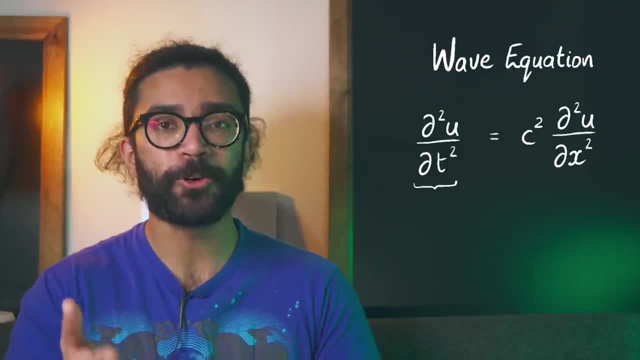 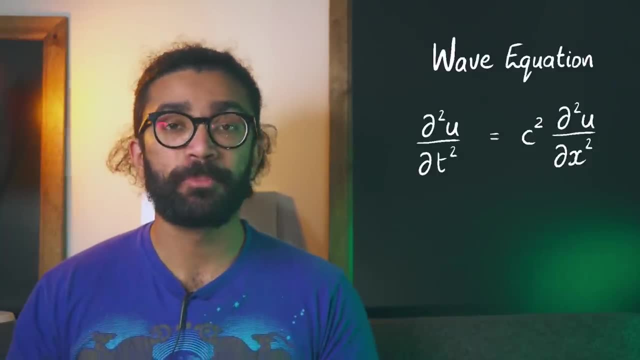 second derivative of u with respect to t. Now, if you don't know what any of this means or want to know more about the wave equation in general, then check out this video up here. But the point is that in our theory of classical physics, which seems to reasonably represent the 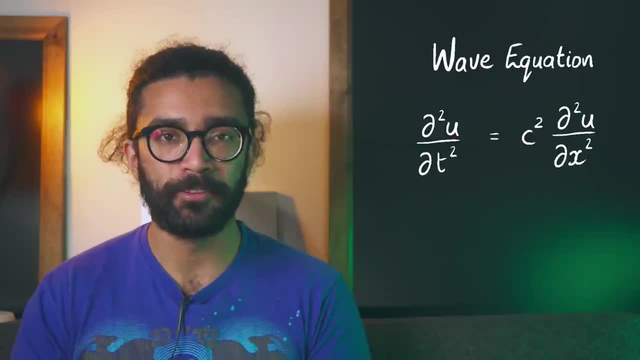 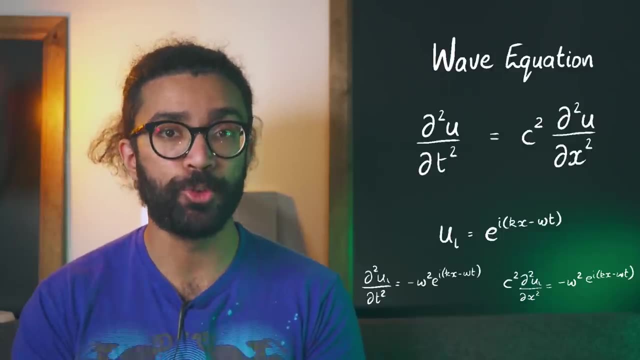 behavior of our universe. any classical waves that can exist must follow this equation. Their mathematical forms must be such that they do fit the wave equation correctly, And this is true for electromagnetic waves such as light water waves, waves on a string and many more different kinds of wave as well. 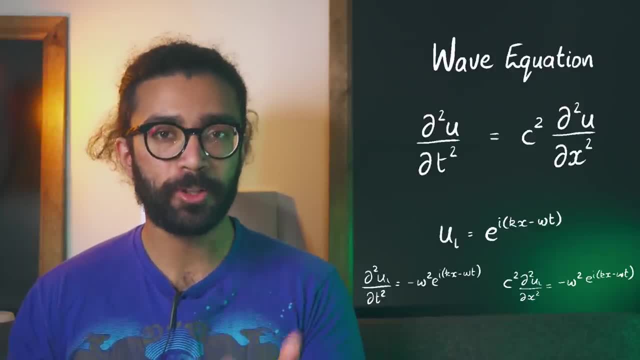 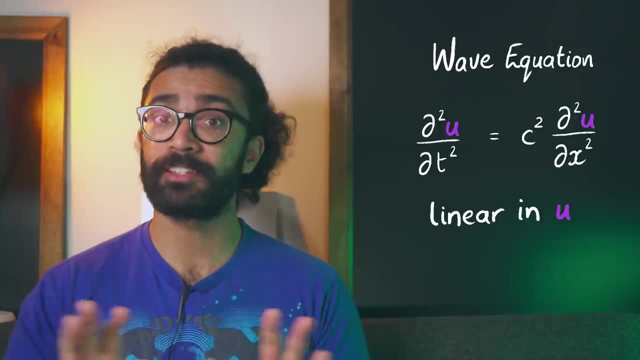 Now, the reason we bring up this wave equation is because we can notice that it is linear in u. What this means is that wherever we see a u in this equation, it's just a single u. It's not u squared or u to any other power or the log of u or e to the power of u. 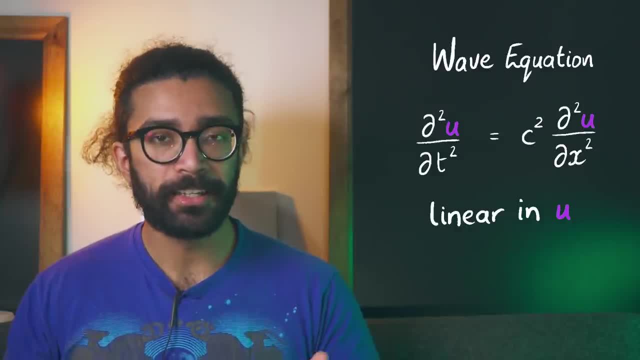 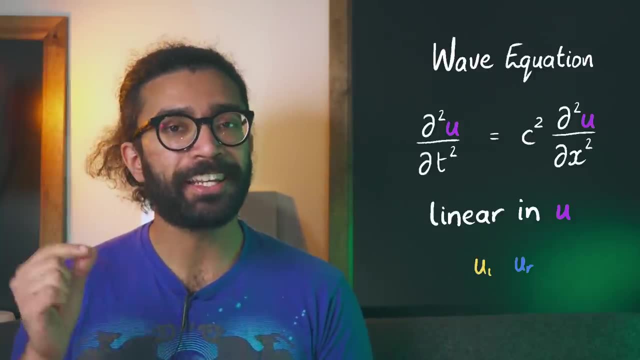 or anything else like that. Because this equation is linear in u, we can take any of the solutions to the wave equation, such as the two wave solutions we saw earlier. we can add them together and the end result is also a solution of the wave equation. 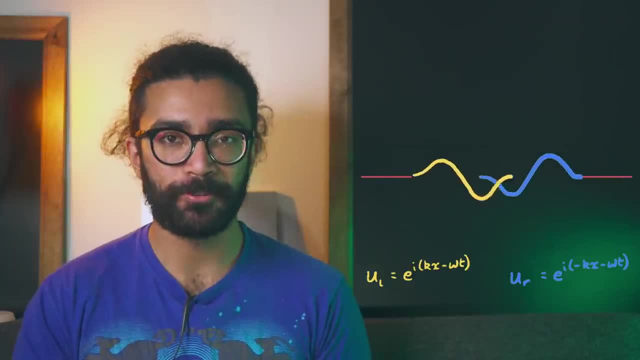 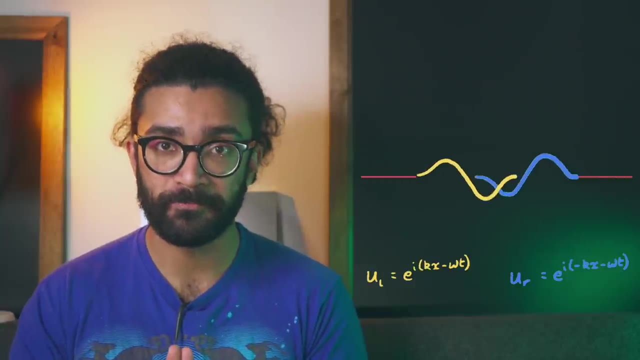 For those of you familiar with differentiation, try taking these two wave solutions, adding them together and then seeing if the end result is another solution to the wave equation. What this means is that just by adding the two original waves we can find another solution. 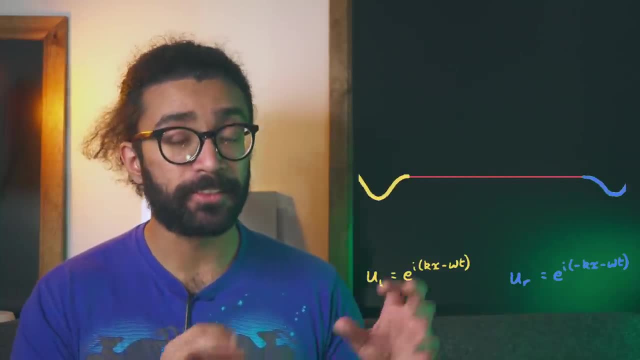 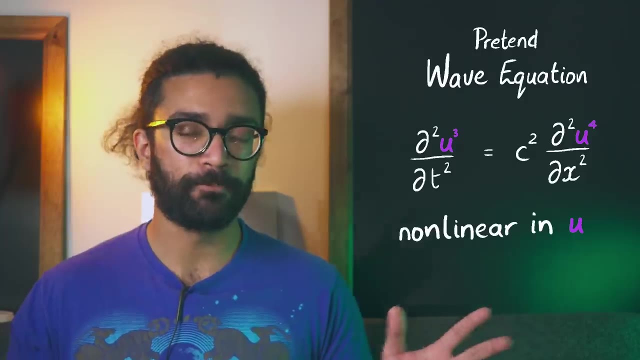 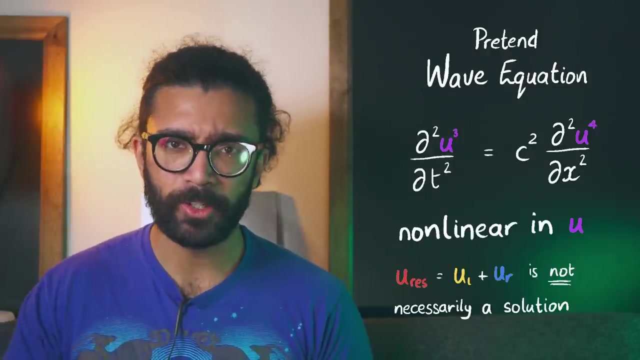 and so the summed or the resultant wave is allowed to exist in this mathematical framework of waves. Imagine changing the wave equation so that it was non-linear and assume that we had found two solutions that worked for this equation. Then a third solution would not necessarily be found. 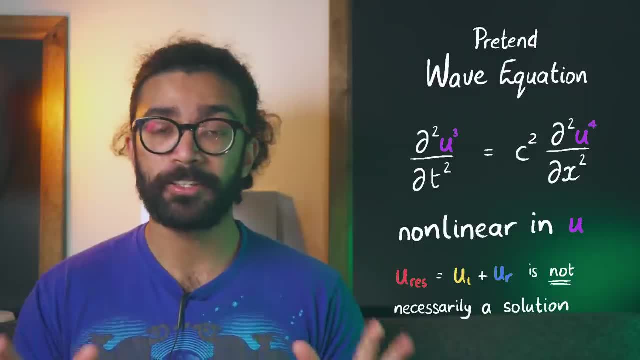 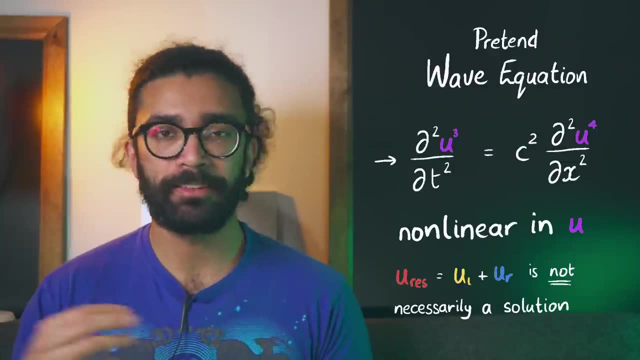 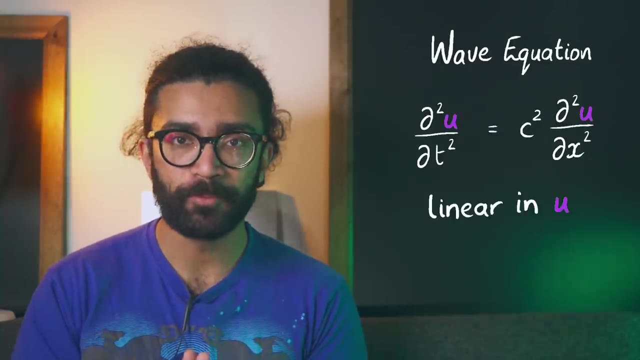 if we added the two original ones together, In other words, if the universe behaved like this in a non-linear way, then waves would not just add together simply by taking their? u values and summing them everywhere. But, as it so happens, the real classical wave equation is linear. 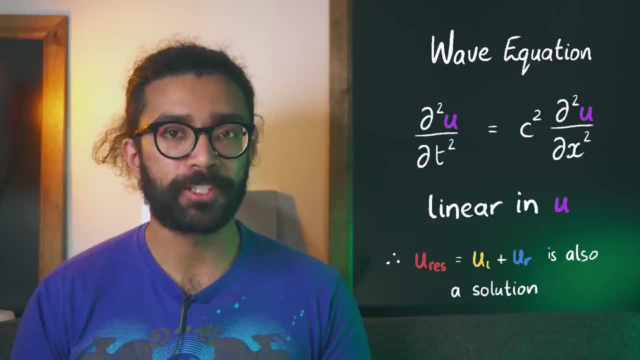 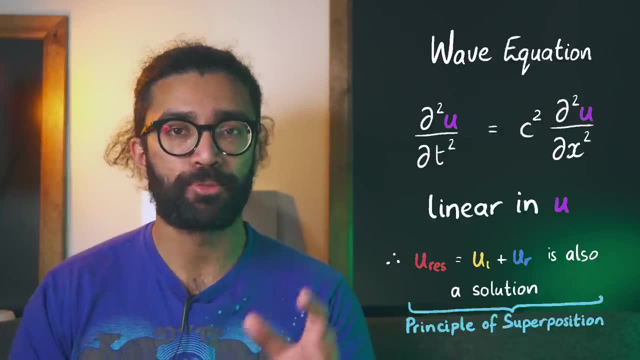 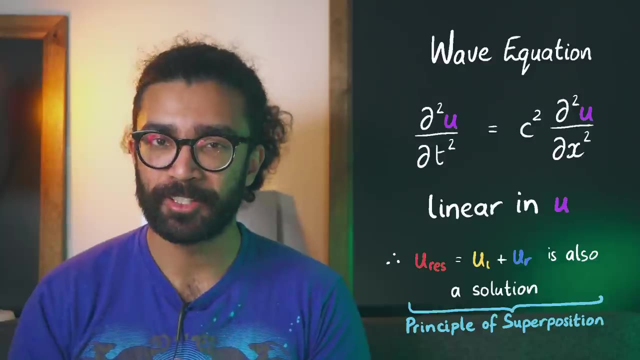 and we can add solutions together to find out how waves combine when they overlap. The property of adding waves together to find an allowed solution is known as the principle of superposition, and it applies to many other linear systems in physics, not just to waves, And as a result of this we can work out quite. 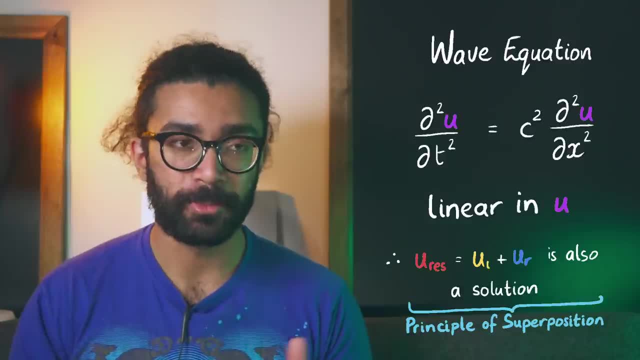 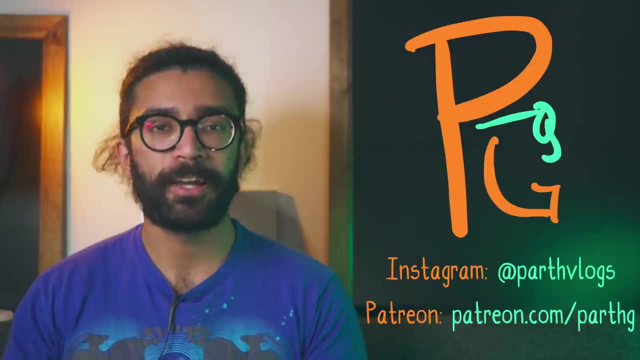 easily what would happen when two waves overlap? We simply take their u or displacement values and add them together, knowing that they will be a solution to the wave equation. Now, with all of that being said, I'm going to finish up here. 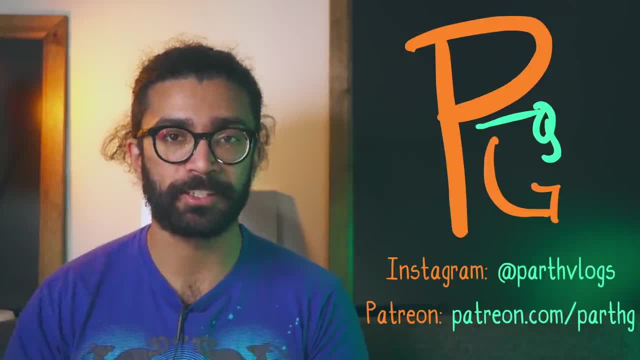 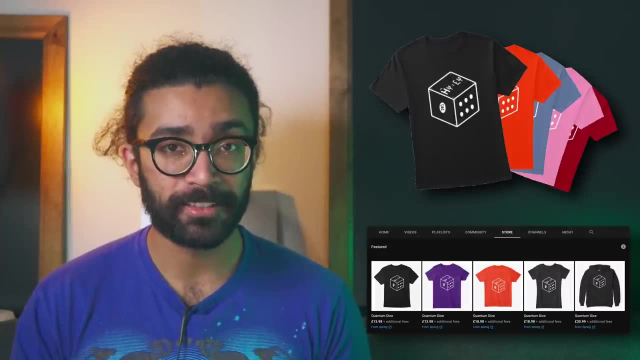 Just a short one for this week. If you enjoyed this video, then please hit the thumbs up button and subscribe for more fun physics content. Check out my merch, linked in the description box below. It features a quantum dice design based on a famous quote from Albert Einstein. Finally, I'd like to say a big